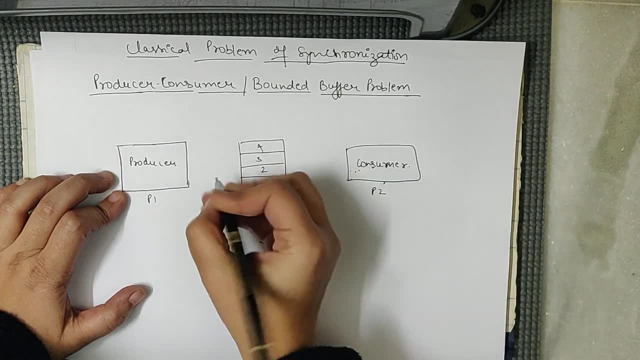 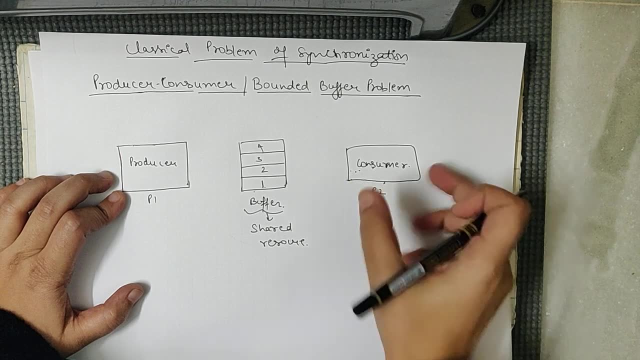 is not so fast that he can pick it. So what will happen? According to producer, that data is just being produced. He is not thinking that consumer has consumed it or not, Because producer and consumer have no interaction. So producer is just doing it. 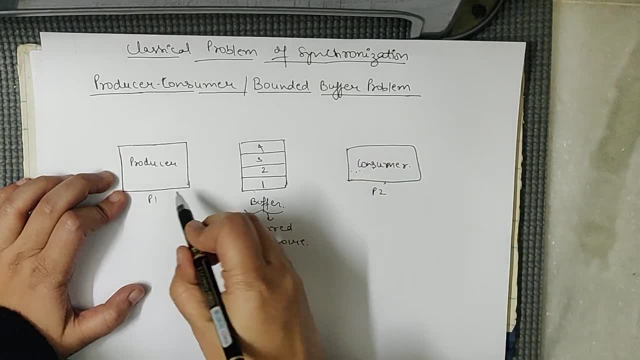 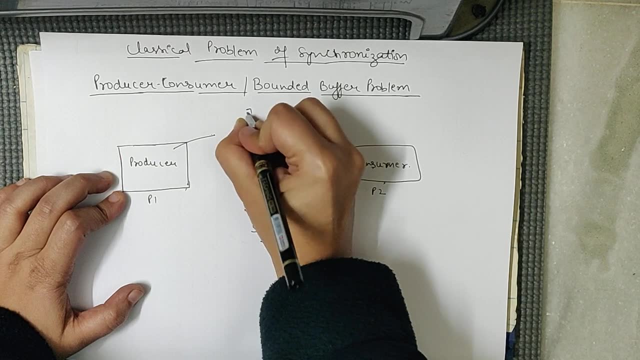 Now what happened One time? it happened that our bucket got full, But producer does not know that consumer has picked data from there or not. So now producer is again putting data. Now what is happening? Data is overflowing. Overflowing means this whole data is lost. 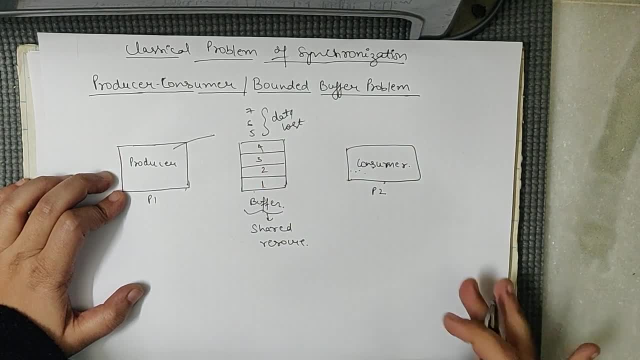 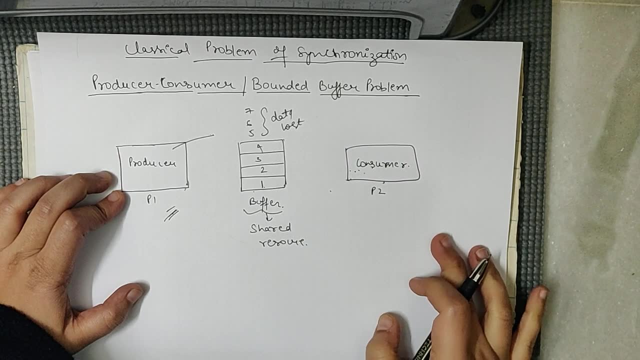 Means consumer has no work. This data is getting lost. Did you understand? This is a problem of producer's side. What is the problem? If our buffer gets full and consumer is not able to consume it with that speed, then data gets lost. 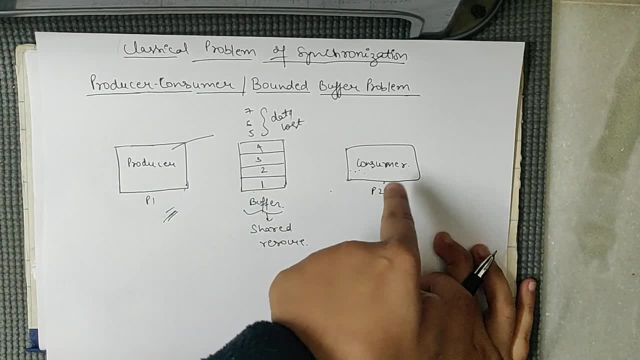 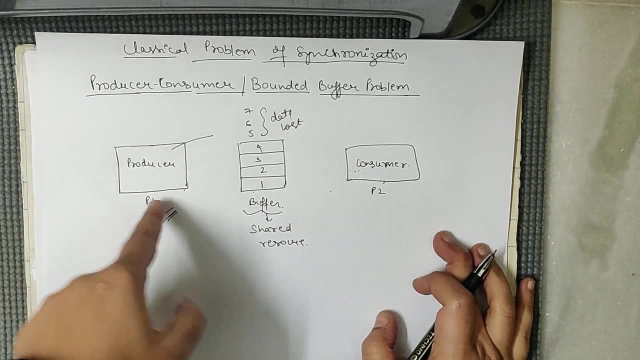 This is a problem of producer's side, Whereas what is the problem of consumer's side? Suppose, consumer has so much speed to consume, Suppose And producer does not have that much speed to produce. So consumer picked 1,, 2,, 3, and 4.. 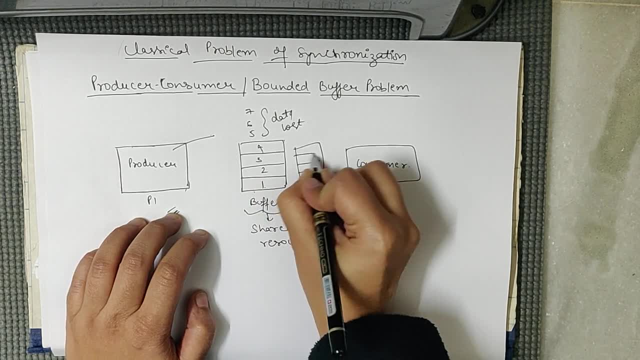 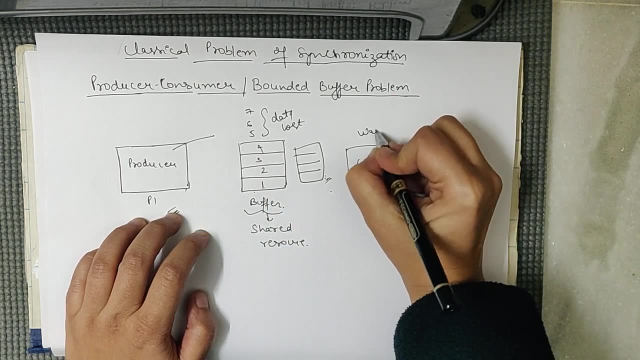 So at one time it happened that bucket got empty. Okay, Producer is not producing with that speed, So now bucket is empty And what is he having to do? He has to wait, Which is also a problem. So this problem, producer-consumer problem- 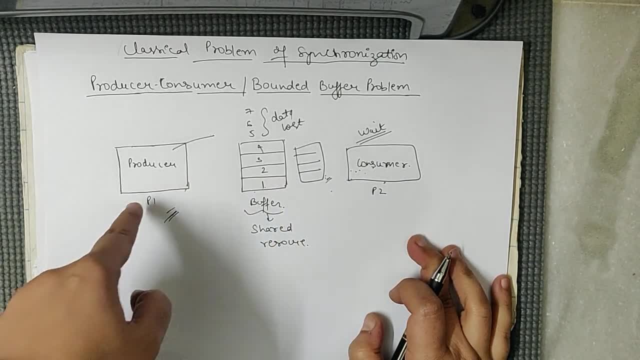 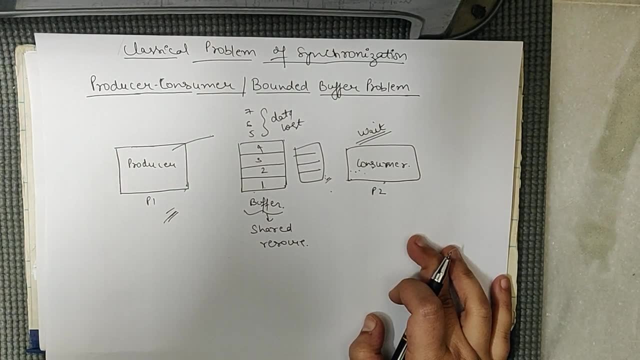 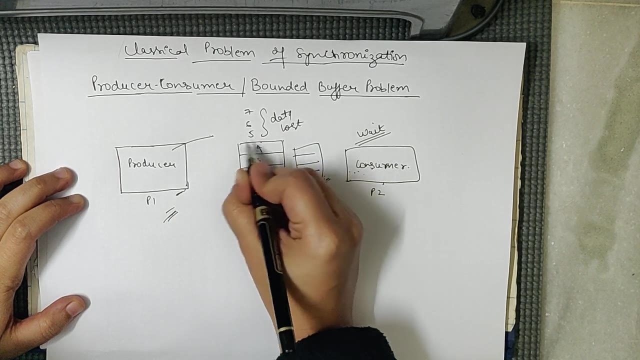 or bounded buffer problem can come from both ends. It can come from producer's end and consumer's end as well. So this is a problem of synchronization. Now, what will be the solution of this problem? We will tell producer that if buffer is full, bucket is full, then he should wait. 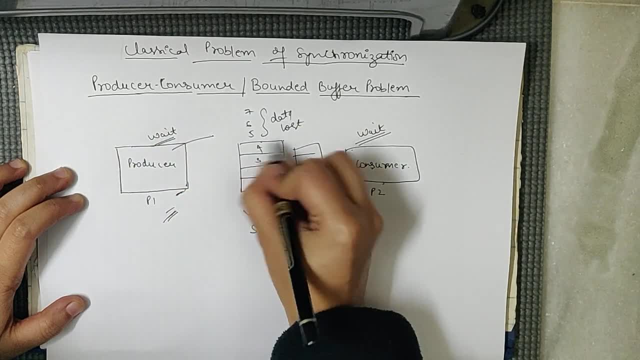 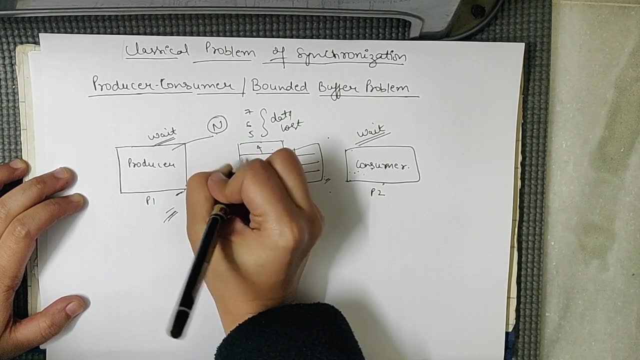 Wait until consumer picks up data item from here. Okay, If bucket is full, then he should wait. If the size of the bucket is N, then if, if the bucket reaches N while putting data, if the bucket is full, then producer has to wait.